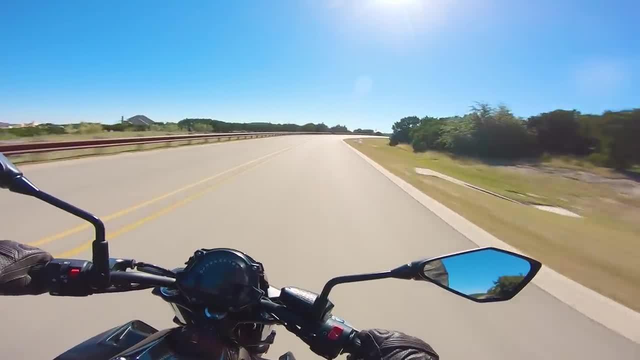 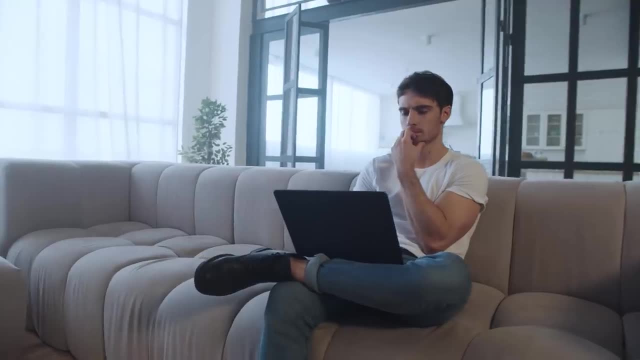 break down a few things you need to know Before you even think about hopping on the bike. and no, it's not going to be riding tips or anything like that. We're mostly going to be clearing the air about a few misconceptions that you might've picked up from watching a bunch of YouTube videos. These are going to be seven. 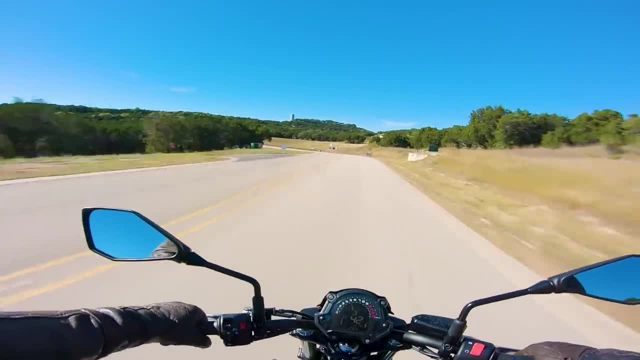 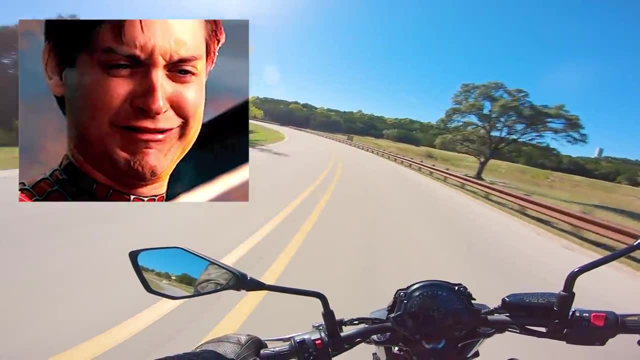 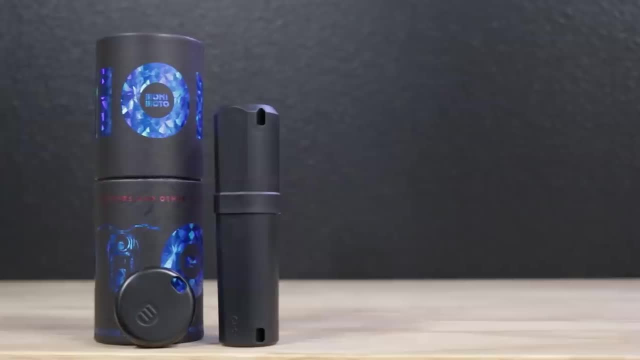 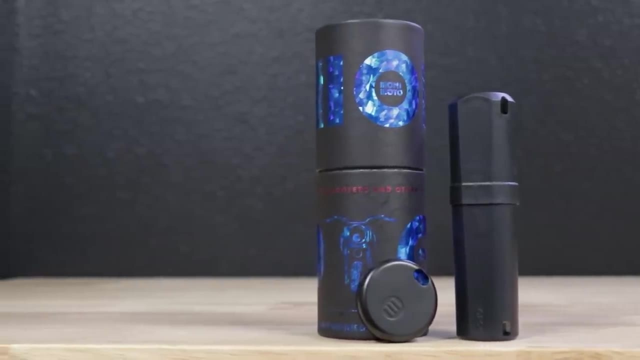 you absolutely should invest in a tracking device, and Monte moto has you covered with some of the easiest motorcycle trackers to install and use. the tracker is super low profile. It doesn't need to be hooked up to your battery, meaning there's no wires to hide, and you can move it from bike to 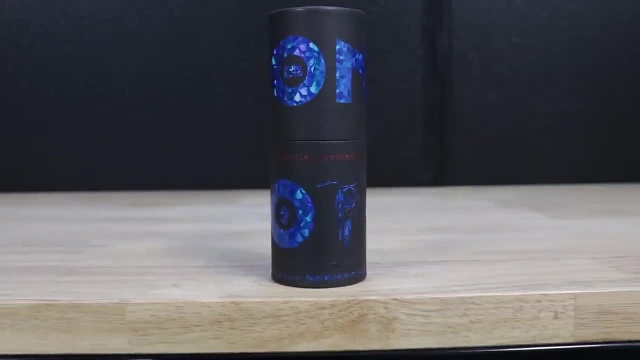 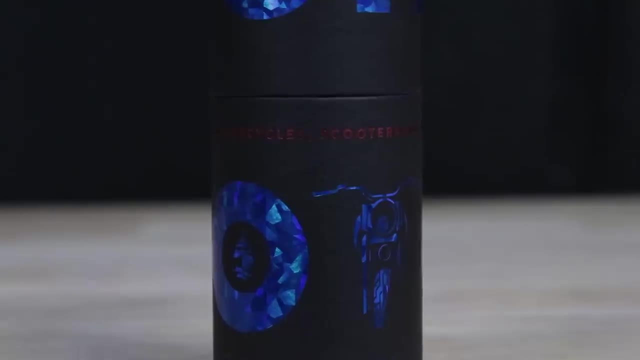 bike Setup is so easy. a boomer could do it. It runs on its own battery that lasts a year, which is pretty sweet. I mean, what was the last time your cell phone made it through an entire day, let alone a year? If you click the link down below and use the code, Yami seven. 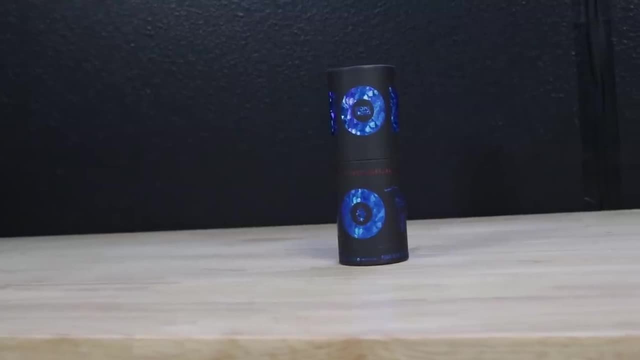 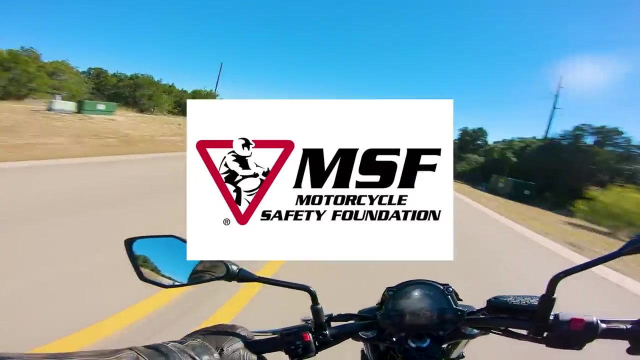 you'll get 7% off your order. If you're a motorcyclist, you owe it to your bike to help help keep it safe. click the link. my dude number seven, the msf doesn't teach you everything. you just finished your weekend at the motorcycle safety foundation course, ran out and bought your. 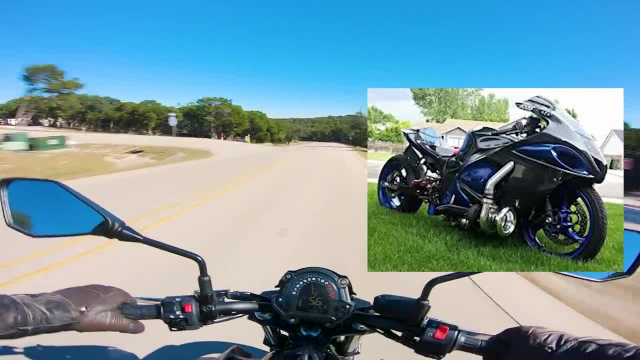 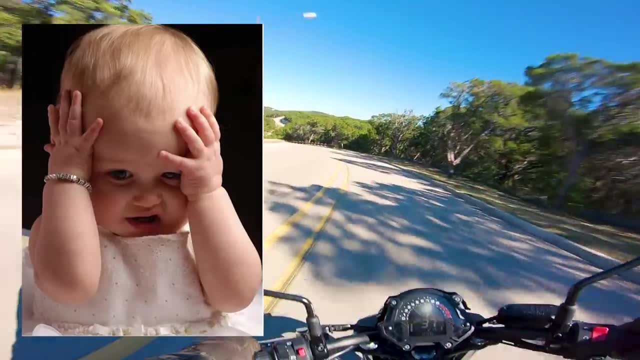 turbo hayabusa. like the good little squid you are and ready to head down to your first ride on the street. the only problem: the driveway out of the dealership is uphill and you need to hang a right on that incline. you search deep in your brain for something that your instructor might have said, but 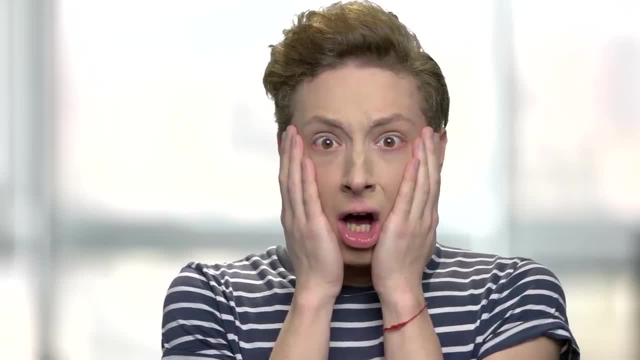 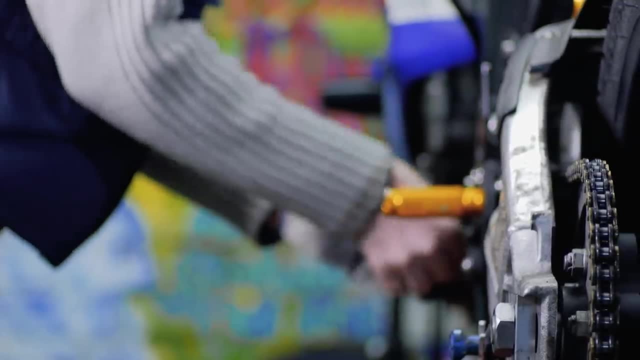 alas, they never taught you that you need to use the rear brake and throttle at the same time and you end up dropping that brand new busa right on the turbo. well, at least you're at the dealership. just get one of the service guys to come pick it up and get it fixed for you. that's right, there's. 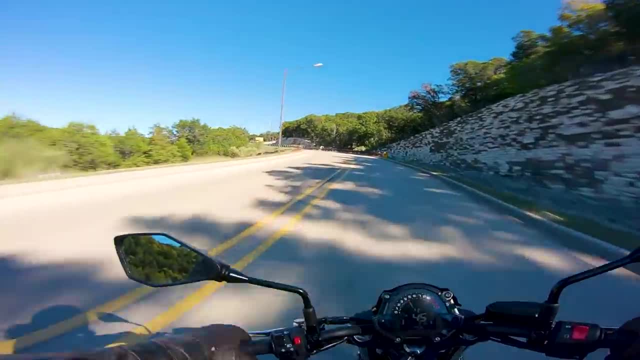 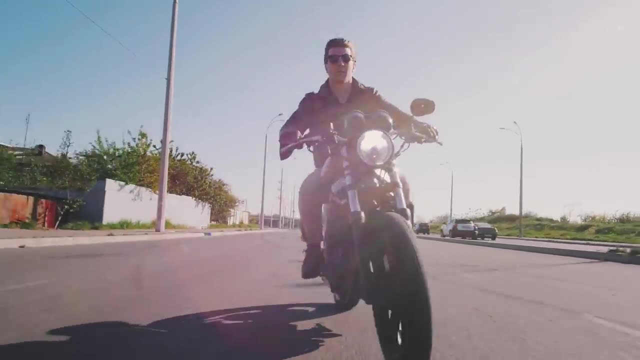 a million little things that you learn as you ride and aren't covered in the msf. why? because the msf is designed to take a person who has never ridden a motorcycle before in their life and teach them just enough to not yeet themselves into infinity. but there's not enough time. in four days you spend. 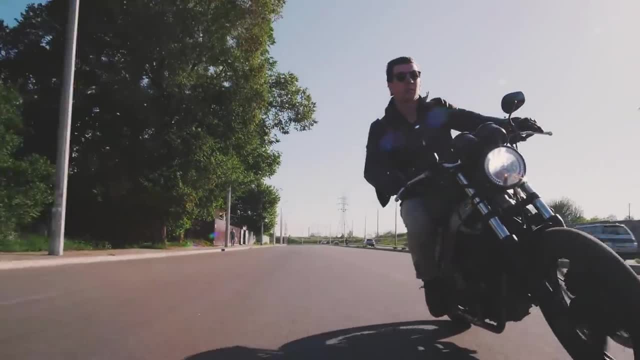 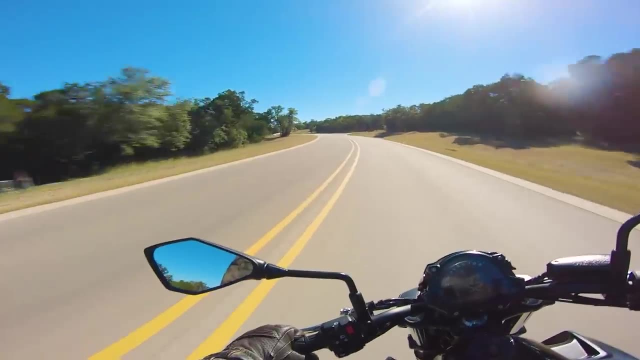 the parking lot to learn how to rev, match your motorcycle and downshifts, or how to pick up your motorcycle if you drop it, or even how to ride in traffic. all they teach you is how a motorcycle works at speeds under 30 miles per hour in a parking lot, and that's just not enough. there's a daunting amount of information that you 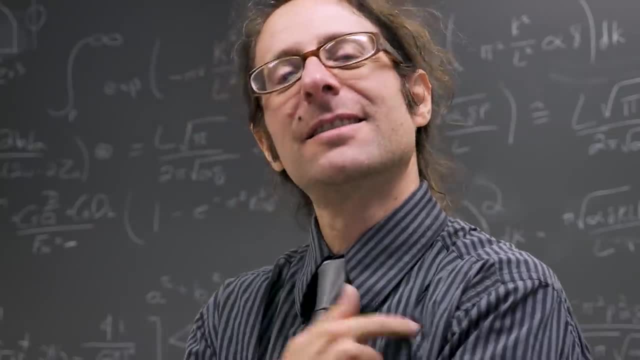 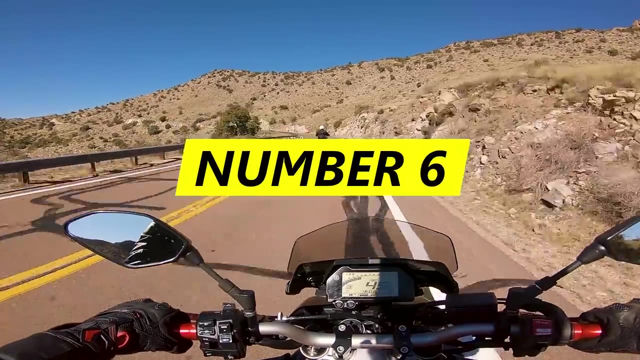 will learn, but it will take time. and in the same sense, don't think that just because you ace the written test and pass the practical test with flying colors that you know everything you'll ever need to know about bikes number six. you're gonna drop your motorcycle literally every. 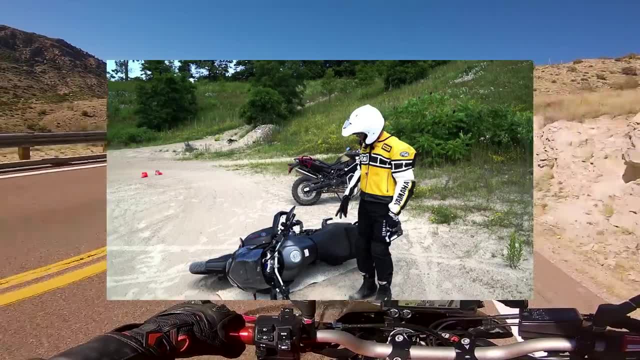 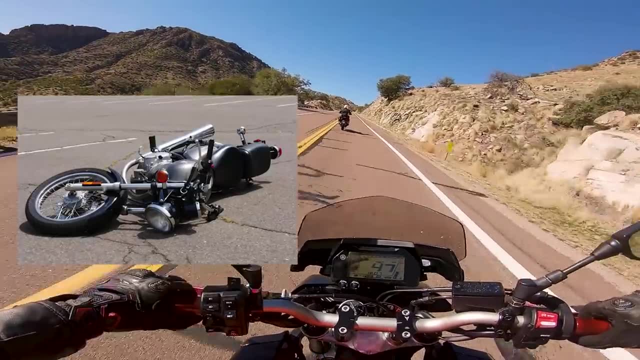 motorcycle is dropped by every motorcyclist. it's inevitability and there's no escaping it, whether you're practicing slow speed maneuvers in the parking lot or your shoelace gets tangled up at a stoplight and you can't get your foot down in time at some. 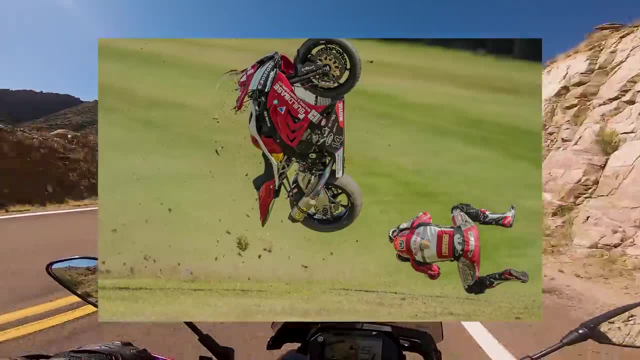 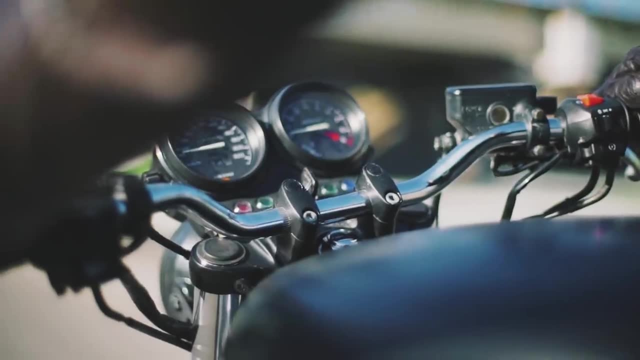 point, your shiny new motorcycle is going to kiss asphalt and come up a lot less shiny and pristine. here's the thing, though: dropping a motorcycle isn't that bad, unless you're really unlucky. you're not going to hurt the bike that badly. you might scuff some plastics, bend your lever or foot. 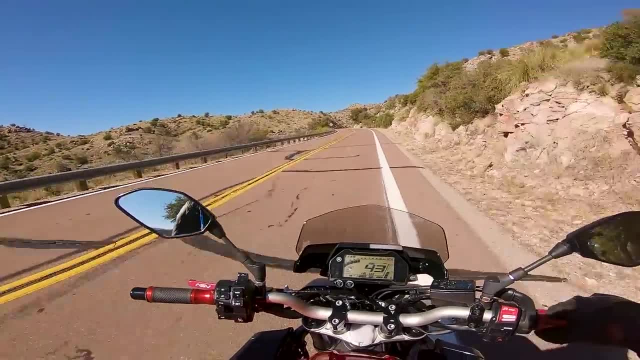 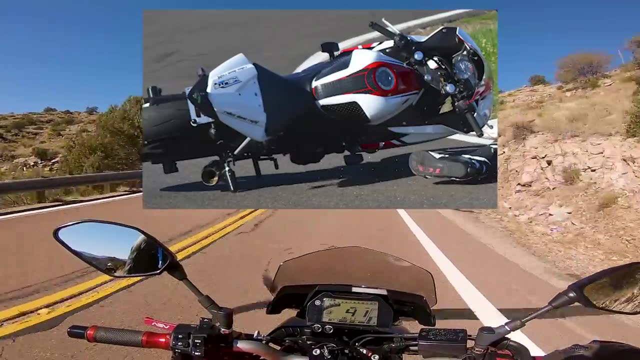 controls and maybe break a mirror, but that's all replaceable. the smart thing to do is prepare your motorcycle to be dropped, including stuff like frames, ladders, case cover and other coverings to prevent damage. they usually all come with plastics like this one, but if you want to get rid of it, you 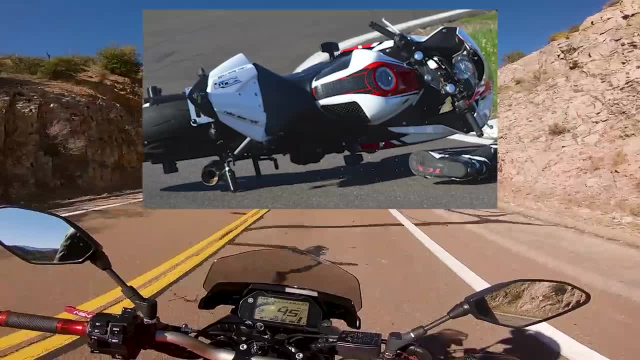 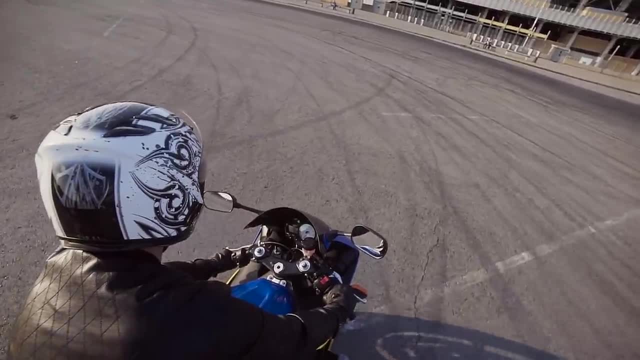 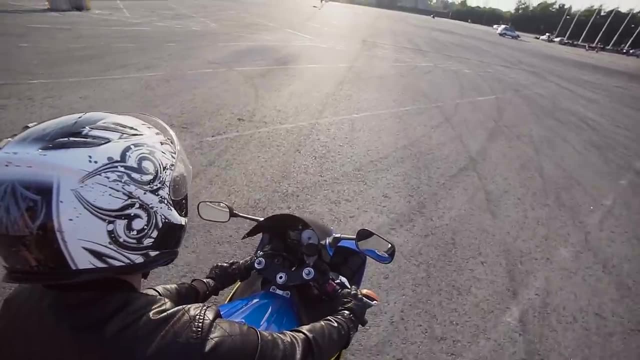 damage, and they're a great way to protect your bike. put it this way, it's cheaper to replace a piece of stuffed plastic than fix a hole in your clutch cover if you drop your bike and you don't have any of this protective stuff. there's a handful of things you can do to repair any of 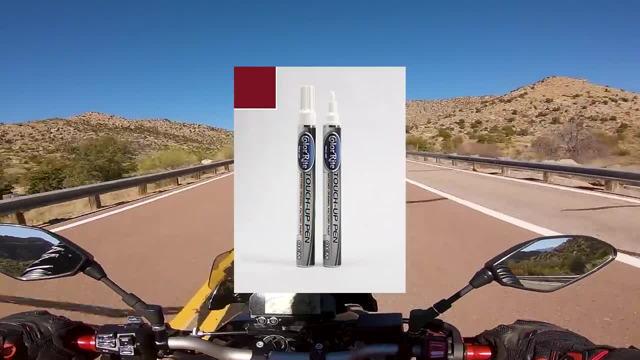 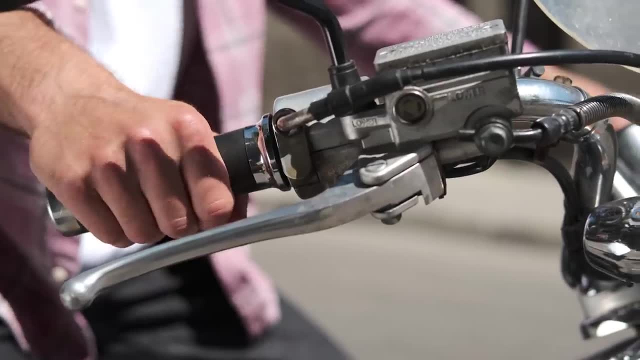 the damage you might incur. first, there's paint pims that can be matched to your bike's factory paint job. it won't fill in any deep scuffs. it will cover up any chips or dings you might get. you can also get a nice set of replacement levers to fix the broken or bent ones. do yourself a. 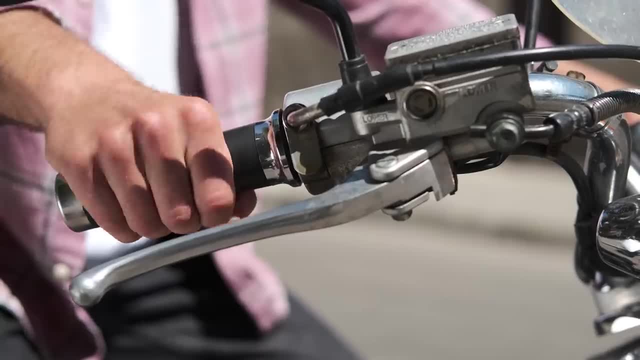 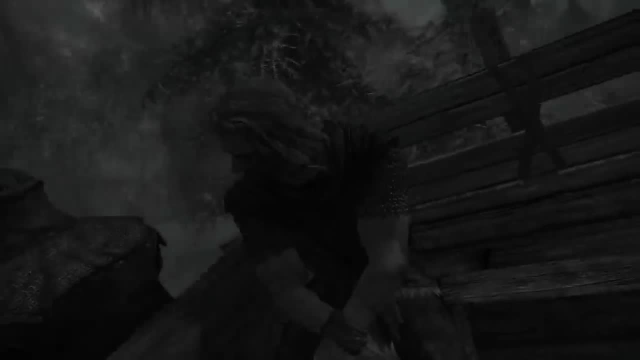 favor, though, and don't buy cheap amazon levers. they work fine, but they look a little crappy and, if it's any consolation, i was literally out earlier today and yeeted my bike probably 15 times on a trail that i was riding on my desert sled because of icy conditions. we all drop our bikes all the. 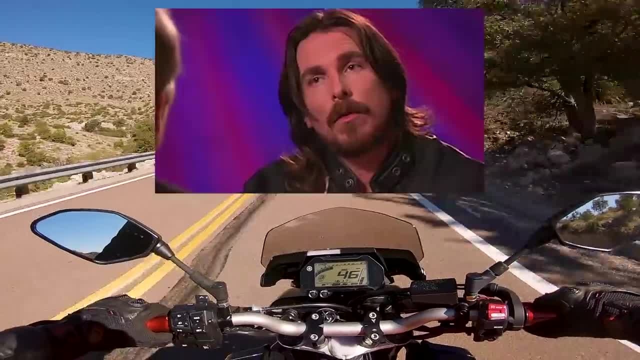 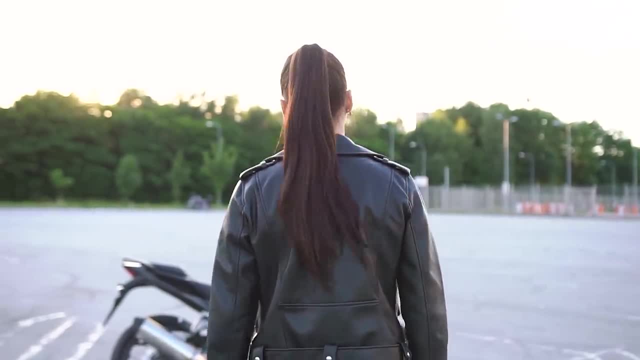 time. number five: gear is disposable. this might be a bit of a surprise, but if you think about it, it makes sense. that motorcycle jacket you just dropped three hundred dollars on won't be the last motorcycle jacket you ever buy. when you ride your bike, your gear is just as exposed to the 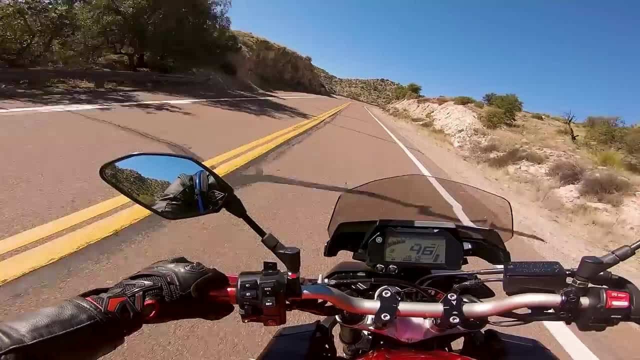 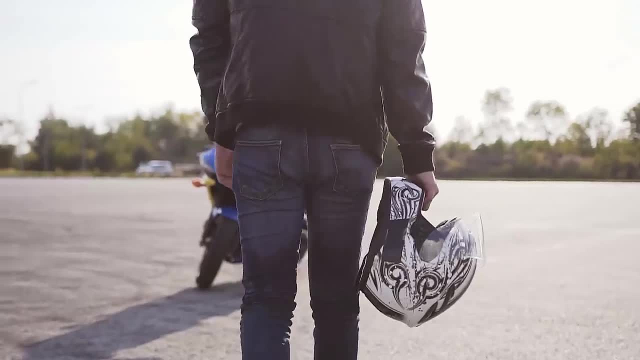 elements as you are. your gloves are constantly touching your handlebars and slowly, friction and sweat will wear them out. your jacket will fade and you might even wear holes in it over time if you don't go down. your helmet needs to be replaced every few years, perhaps sooner if you sweat a lot. 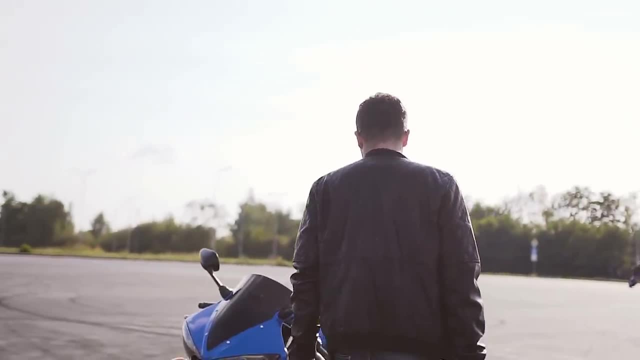 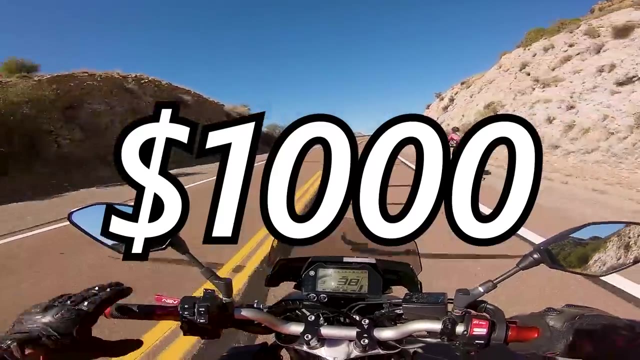 or wear a lot of makeup or hair gel, but you can always swap out the insert foam. however, just because your gear wears out doesn't mean you should cheap out and get lower quality stuff to save a few bucks. you should expect to spend around a thousand dollars on a full set of very 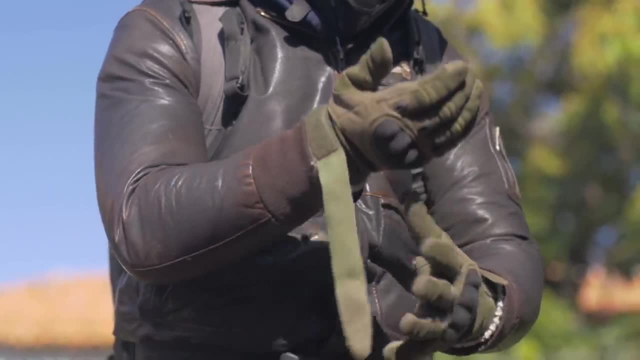 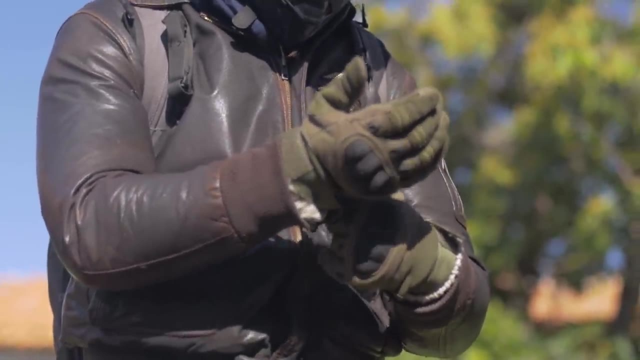 good gear to get started, including a jacket, helmet, gloves, boots and maybe even riding pants if you're so inclined, and that gear should last you at least two years. after that, though, your jacket might be getting stanky, your gloves might have holes in them, and your helmet 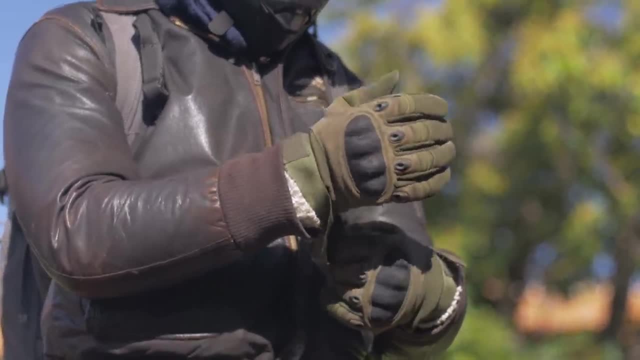 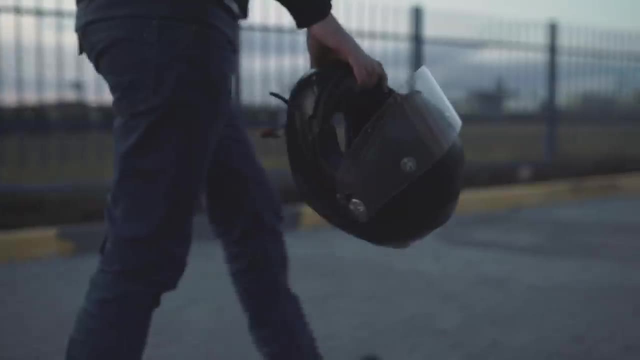 might not be as safe as it used to be that, or you just might want to replace or upgrade your stuff to nicer stuff. expect to spend an additional 500 a year on replacement gear, sometimes more hell. I'm very vain and I love buying new gear to look fresh. also, if you do end up going down most. 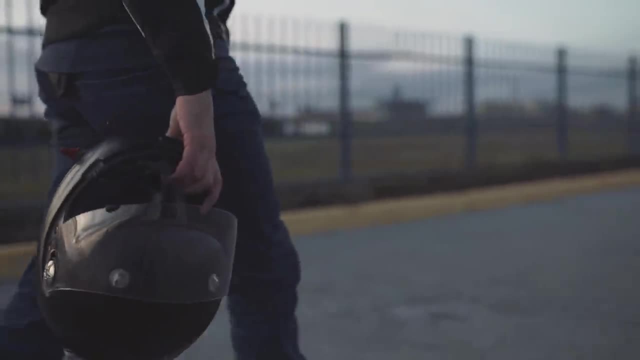 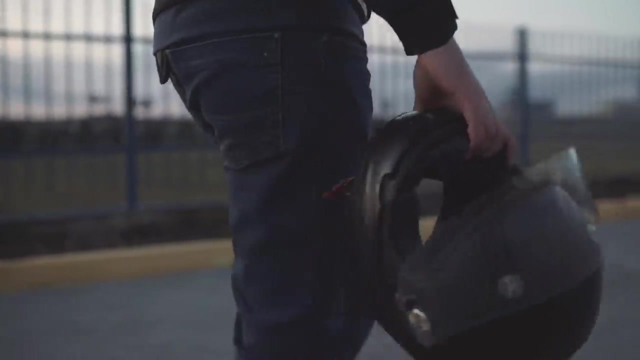 insurance policies will have some considerations for replacing your gear, so don't worry about saving it. unless it's a track suit, this gear is only designed to survive one impact. Papa yams crashed in his track suit at least five times now and it's still good. number four, your motorcycle is disposable. I'm just kidding, it's. 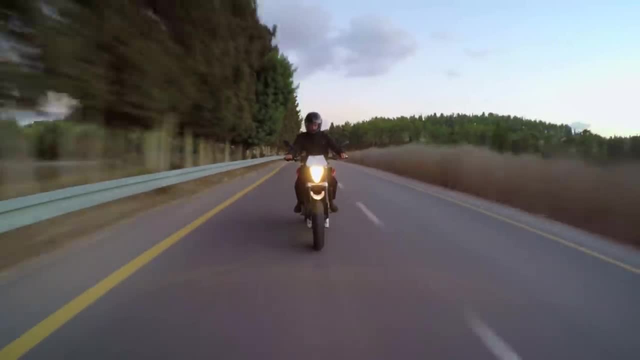 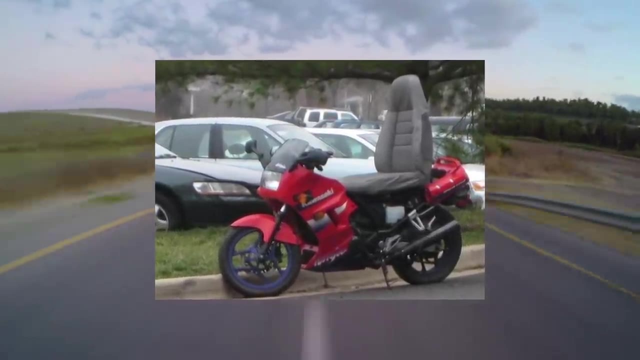 not disposable, but you probably won't keep your first bike heck. even your second, third, fourth, twelfth or whatever. the motorcycle you're riding right now probably won't be the motorcycle you keep for the rest of your life. there's a lot of reasons why you might bin it, you might outgrow it. 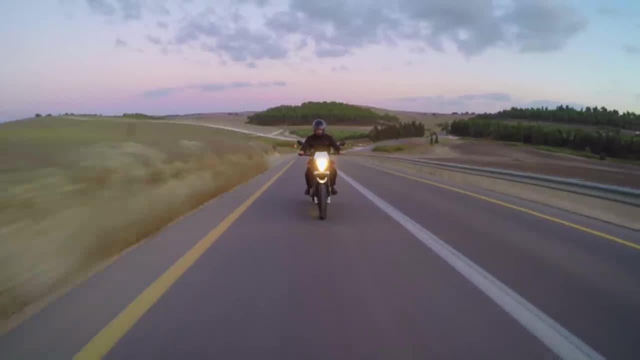 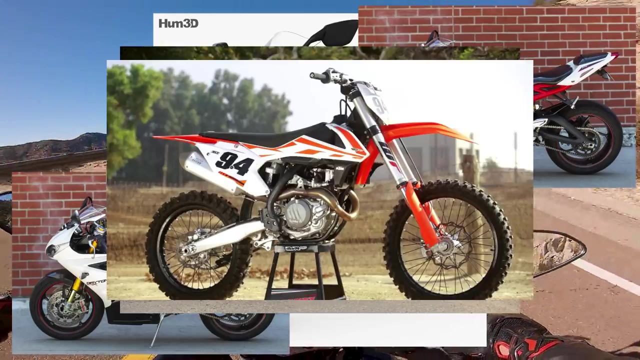 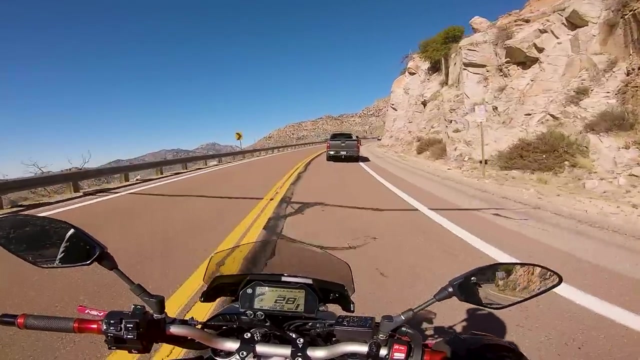 your taste might change. whatever it is, you should expect to own multiple motorcycles throughout your riding career. look at me. I had an R3, three different Daytonas, an FZ09, my desert sled, my KTM dirt bike, my Hayabusa, the RC390. they just come and go. even Spite's been through about six different motorcycle in as many. 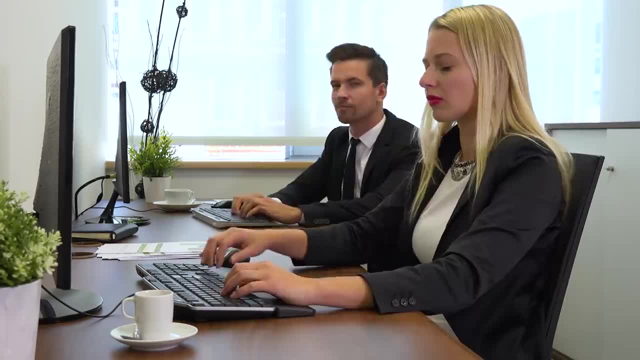 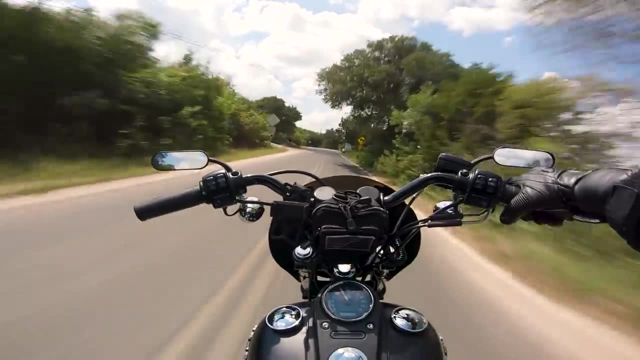 years. it's important to remember this because you might be sitting at your computer right now thinking to yourself that all you want in life is a brand spanking new R1. but you might ride your buddies Harley and realize that you like a relaxed riding position, lack of power and boomers coming. 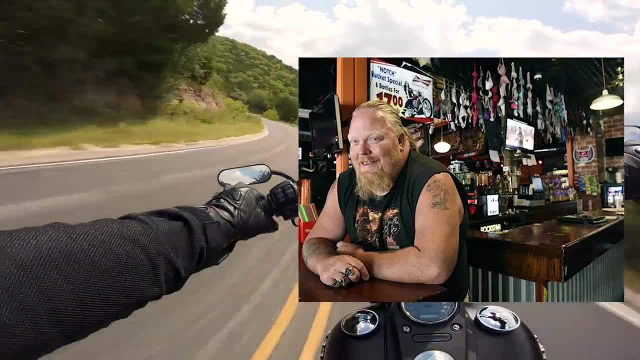 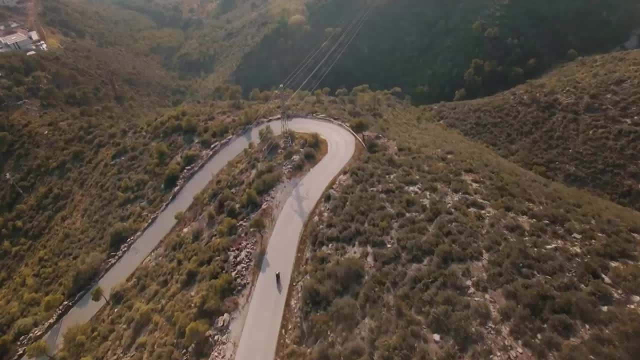 up to you at gas stations wanting to talk to you about how they themselves have a 31 Road King Mega Glide, power cam screaming Eagle hog back home and you might really need to get yourself a real bike approach motorcycling with an open mind. you'd be surprised how many there are. 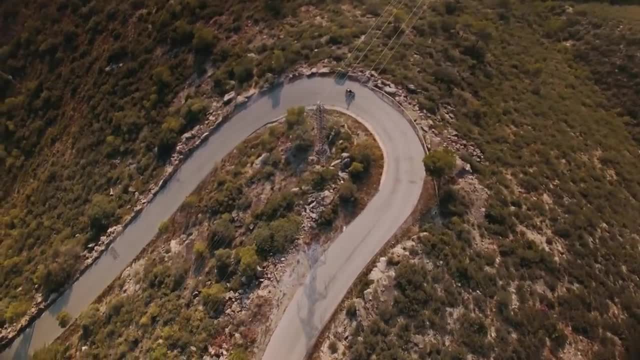 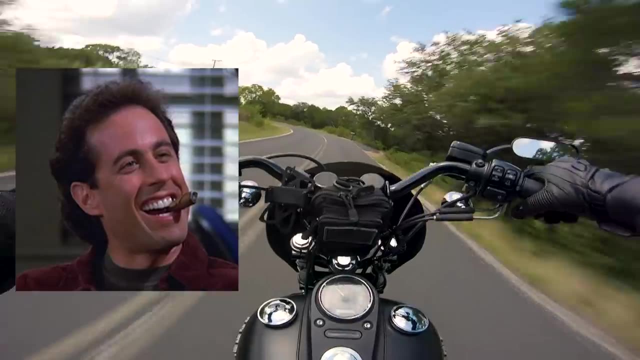 out there beyond the streets, and I mean that literally there's track riding, road racing, trail riding, scrambling, adventure, riding motocross- if you can think of it, you can probably do it on a motorcycle, and it turns out they're all pretty fun. number three: nobody cares that you ride, you might. 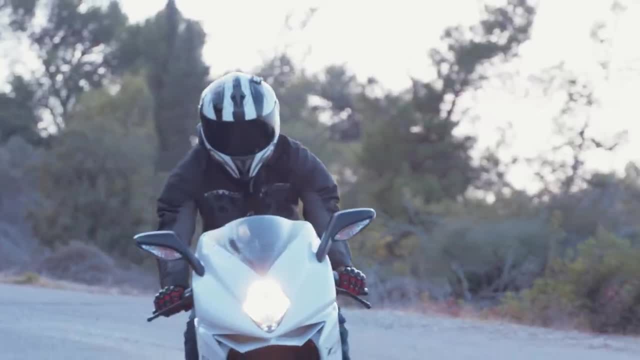 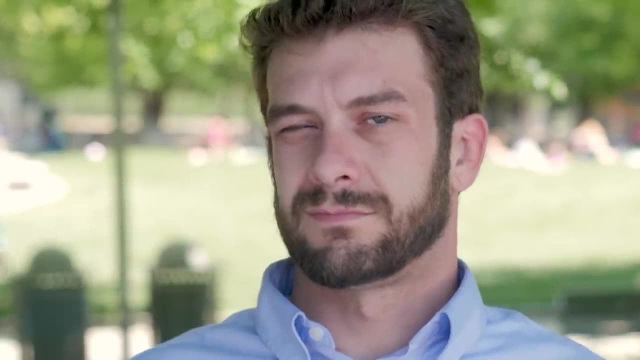 be thinking to yourself that getting a bike will be an instant conversation starter, like you show up to a bar, plop your helmet down and everyone will want to come up to you and talk to you about your bike, bro. most the time even other bikers don't care, they might nod to. 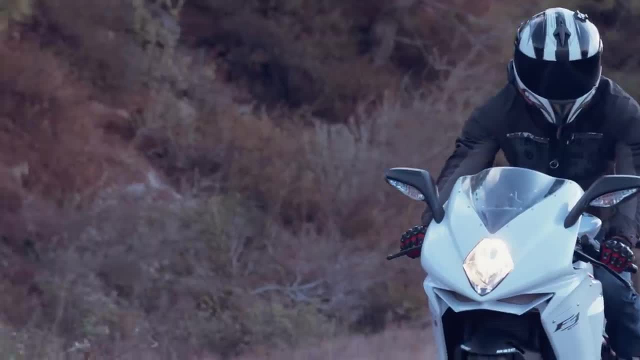 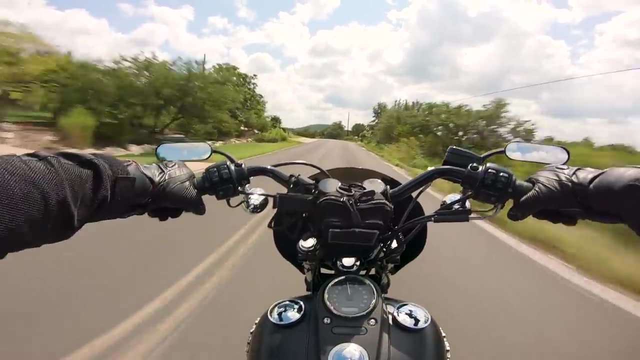 you or wave as you pass by, but chances are they're not going to walk right up to you and ask you about your bike, unless you're currently sitting on it, which would be weird. motorcycle parking is typically on the street, so I'm not sure why you would be out to ride your bike in the bar, but hey. 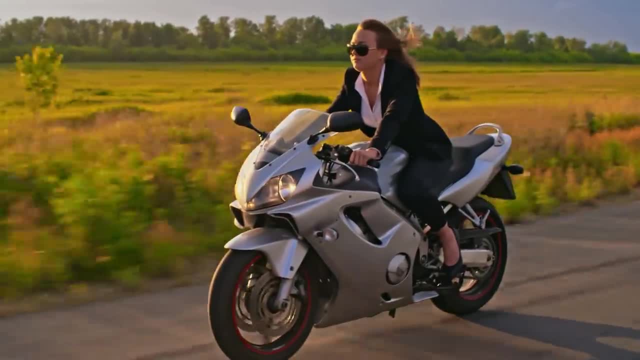 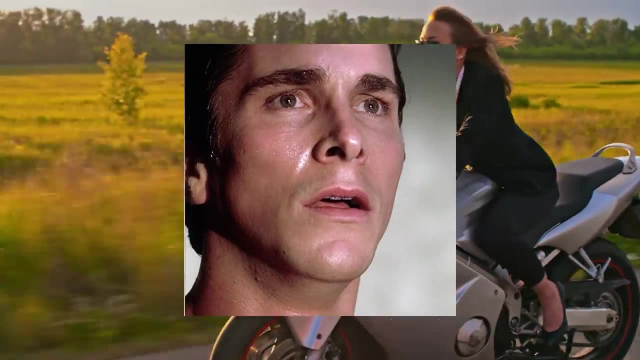 you do you? the only exception to this rule is if you're a woman. if you're a woman and you ride a motorcycle is coming up to you and asking you what about your bike and trying to Mansplain Something to you. I see it all the time and it's super cringe-worthy. guys, if we want to encourage 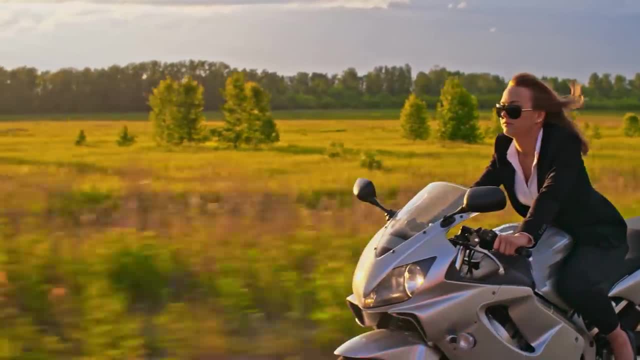 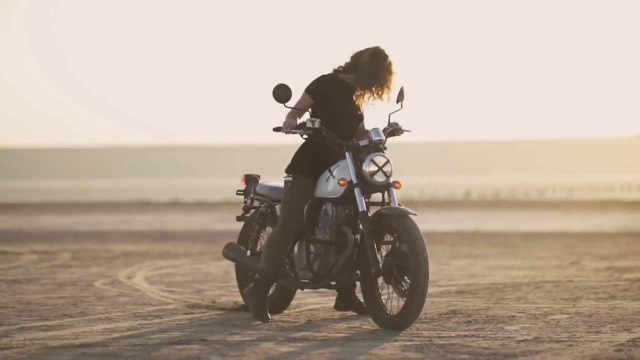 more women to ride, the first thing you might want to try is leaving them alone and not trying to get in their pants merely for the fact that they have two x chromosomes and two wheels. just act like a normal person. it's not that hard. also, chances are. if you see a woman who rides, she 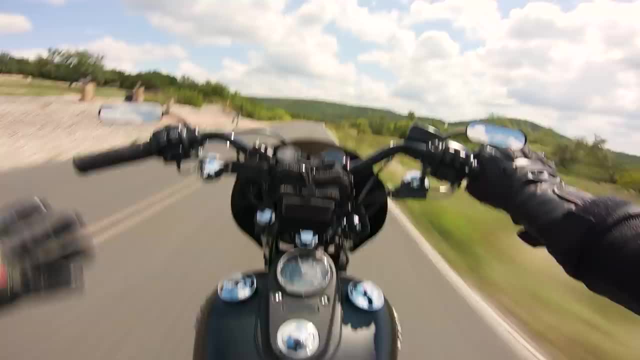 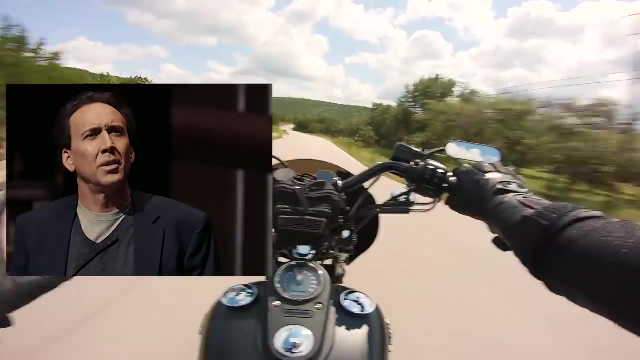 probably knows more than you. so don't try to impart any unsolicited knowledge. hell, don't impart any unsolicited knowledge on a dude rider either. number two: most motorcycle crashes, only vehicle. Why does that matter? Well, think about it for a minute. If a motorcycle wrecks and no one 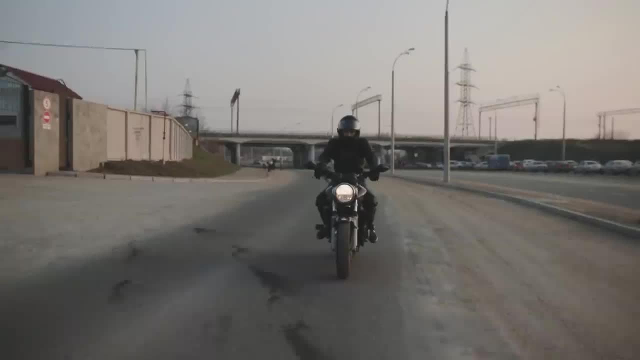 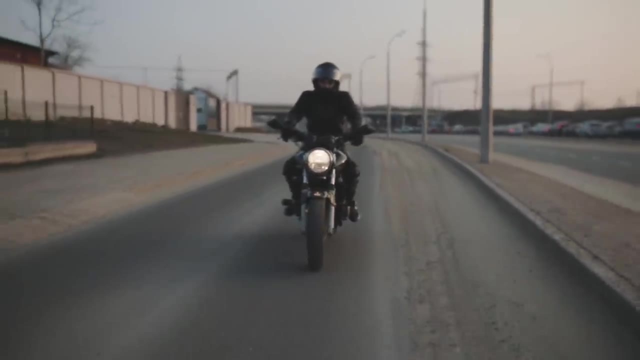 else was involved, that probably means that the motorcyclist is to blame. Usually, the prevailing cause of a motorcycle accident is speed. A squid is out there trying to drag me around a corner on their favorite back road, critically, miscalculates the corner and their speed or ability and ends up. 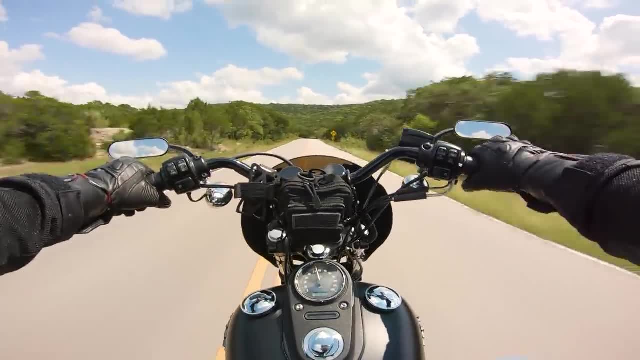 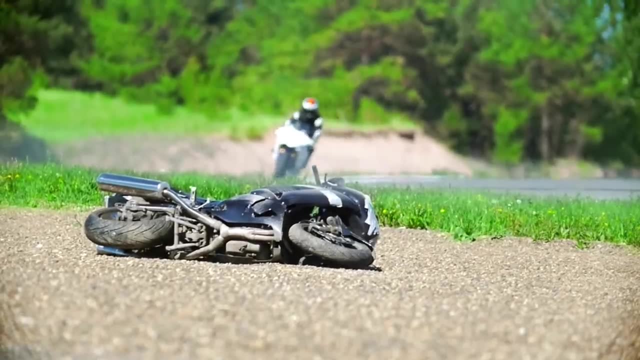 eating themselves right into a tree. When you're out on the road, the most important thing to remember is you have no safety net On a track. there's massive runoff room, groomed infields that don't have hard immovable objects for you to hit, and the tracks are kept clean of stuff like 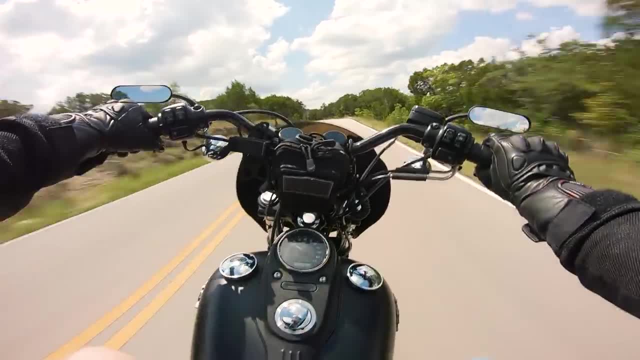 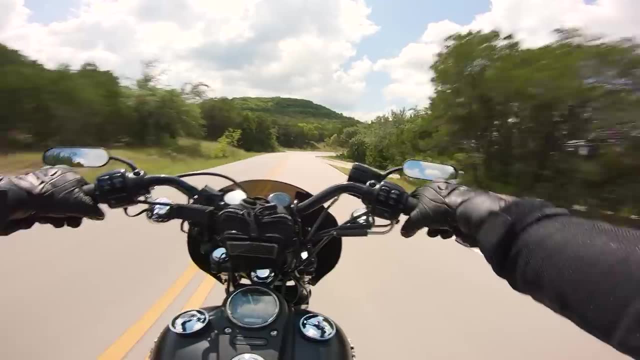 gravel, sand and other obstacles, for the most part On the street. no one's out there keeping gravel off the road, making sure the shoulder isn't covered in broken glass or used needles or making 100-foot deep runoffs so you can recover. Ride your own ride, meaning you're not. 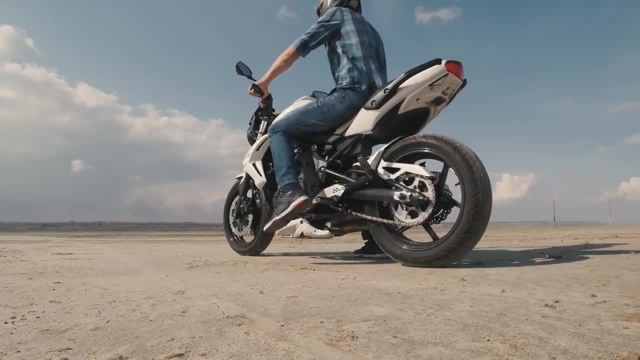 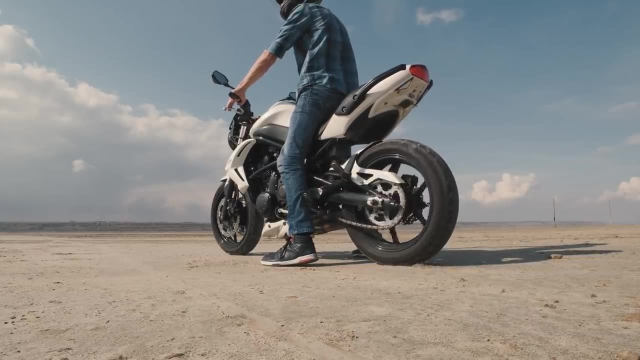 pushing or test the limits of your motorcycle. Keep your speed to roughly around the posted speed limit so, just in case something comes up out of nowhere, you can react. Remember 99 times out of 100, if you go down on the road. 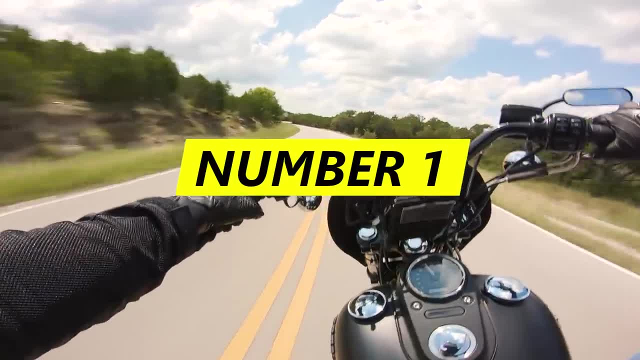 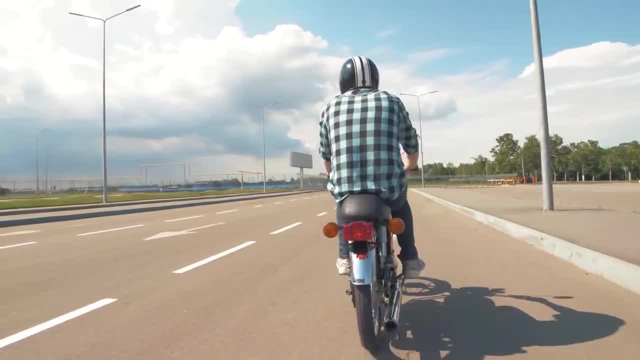 it's kind of a problem Number one: your motorcycle will not replace your car. This is one of the things that every motorcyclist learns over time, but it's best to just rip off the band-aid now. Occasionally I'll see some squid down in the comments- suggest that they might trade in their car. 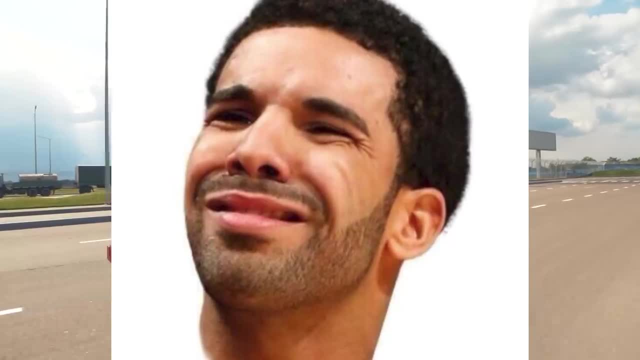 and, with all the money they make, run out and get the motorcycle of their dreams. This is a horrible idea. First of all, how are you going to get your groceries home? You might be able to balance one bag on your gas tank or fit some into the saddlebags, or 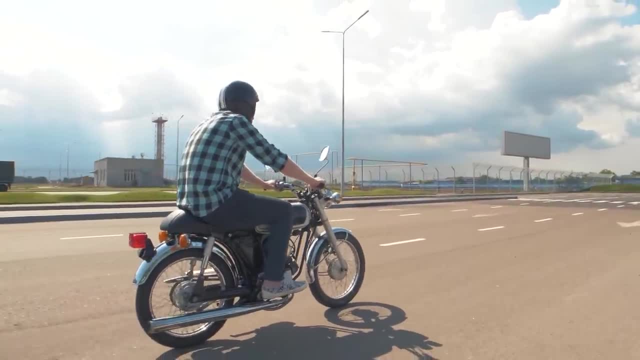 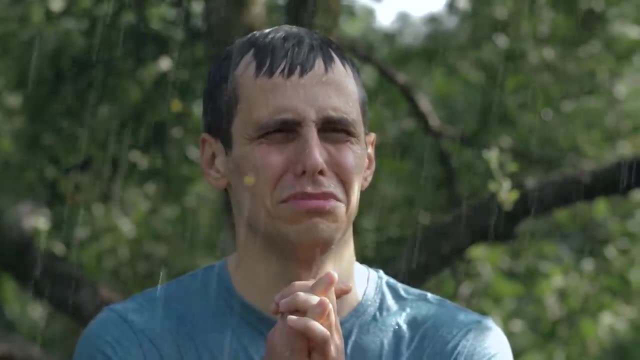 top cases, but it's always easier to run errands in a car. Also, what happens if it's raining? Some new riders will go out, no matter what the weather is like, but trust me that that will fade over time and eventually you're going to get real sick of having. 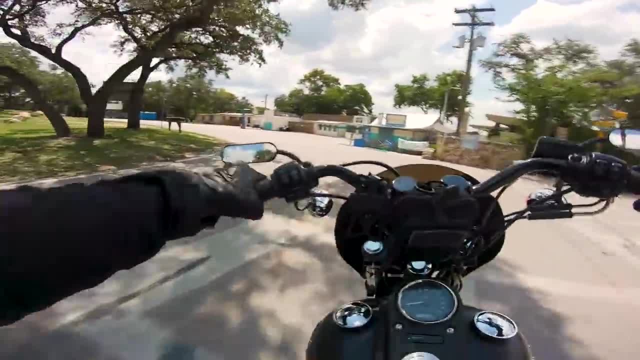 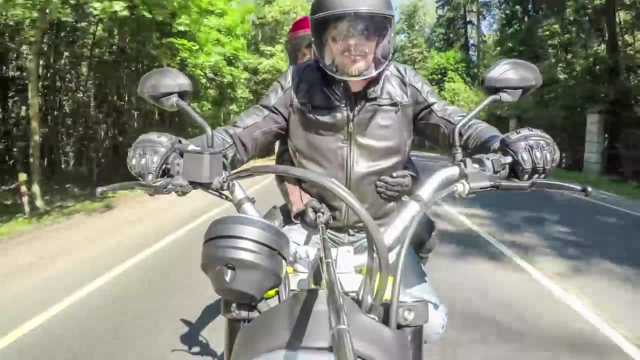 to pack your office clothes in a trash bag and change in the bathroom when you get there? Also, what if you have a date that doesn't want to ride on the back of a bike? That might be a deal-breaker for some, but for others you're probably going to want to wish you had a cage around to drive. 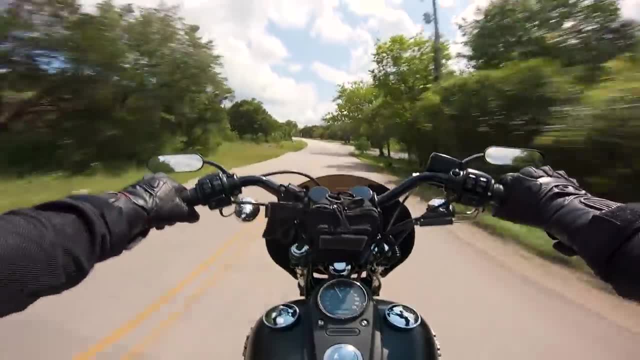 Lastly, an unfortunate reality is there will come days where you don't want to ride your bike. The weather might be perfect, but you just might not feel like going through the whole rigmarole of putting all your gear on the bike. You might not feel like going through the whole rigmarole of putting all your gear on the bike. 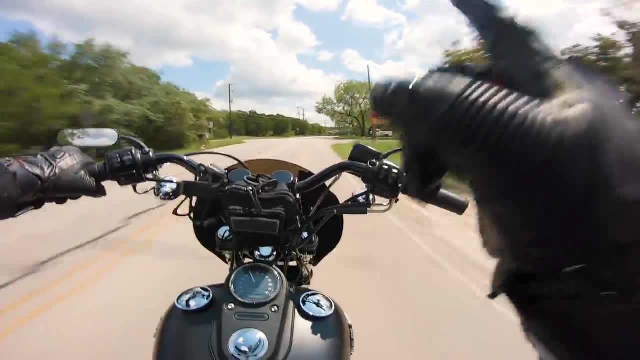 You might not feel like going through the whole rigmarole of putting all your gear on and just take the car to go do something. Just remember that for most people a motorcycle is just a toy. You've made it to the end of another Game & Noob video. 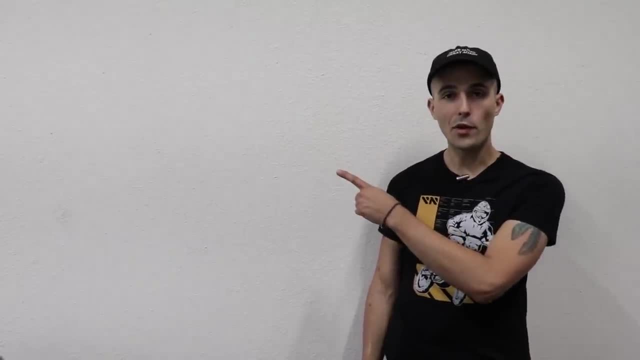 Aren't you a special cookie? Well, I'll tell you what I got a gift for you. Click this right over here. You keep watching yourself some of my videos. Got some cool ones in there. Got some memes, Got some awesome content. I don't like the way this one's feeling. I'm going to try it again.